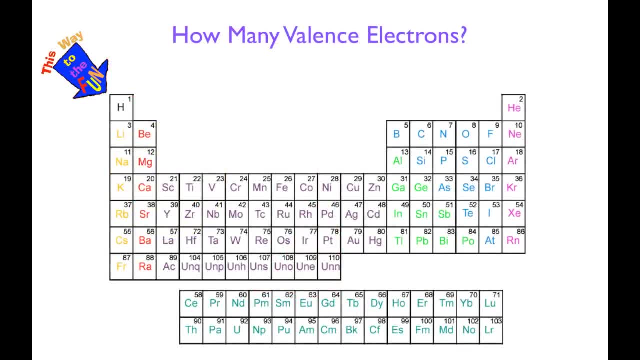 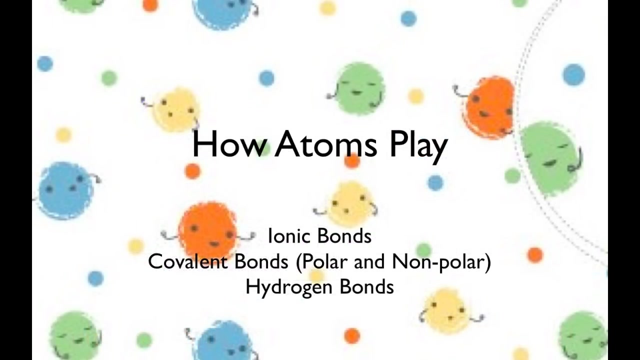 want to feel just like a noble gas, even if you're not So, if you recall the periodic table and the valence electrons, it's pretty easy, because all you have to do is look straight down in these groups or the columns and you see how many valence electrons a particular element will have. That's going to make it a lot easier. So the periodic table is your friend, whether you want it to be or not. It's going to simplify your life. Trust me on this. We're going to look at different ways that atoms play together ionically covalently, and we're going to look at different ways that atoms play together. 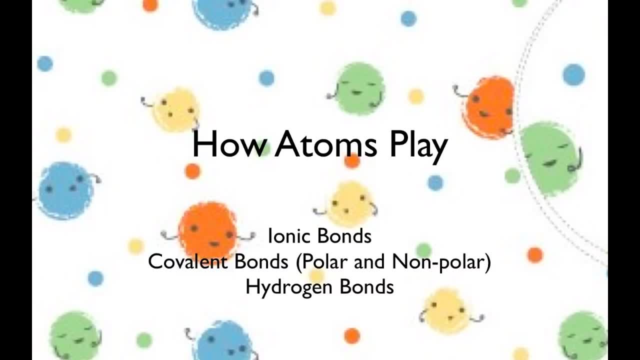 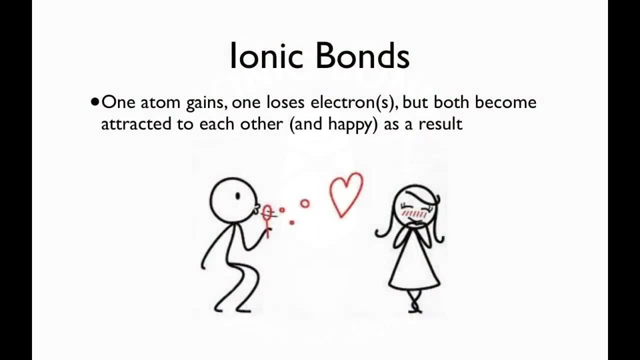 We're going to look at hydrogen bonds. They're actually very important in biology because they hold a lot of really important stuff together. First bond we're going to look at is the ionic bond taken, not shared. It's so dramatic. In ionic bonding what's going to happen is one atom is going to donate one or more electrons And when that happens it's going to gain a positive charge. We're going to see why, Meanwhile, another atom is going to receive one or more electrons and it's going to gain a negative charge. Now here's. 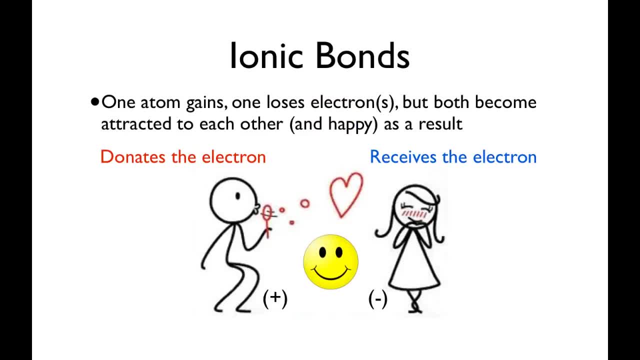 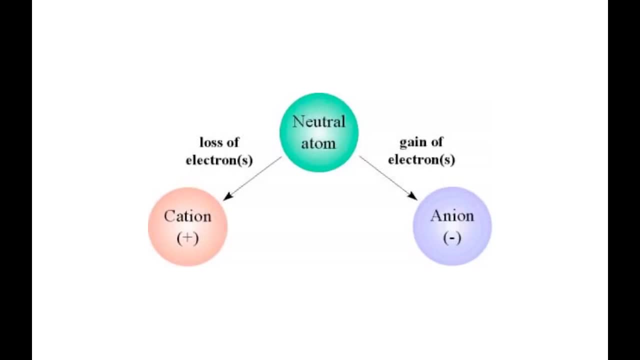 the key in chemistry: opposites attract. So it is the attractive force between the positively charged ion and the negatively charged ion that holds the whole thing together. That's the bond. So in their elemental state, that is when you look at the periodic table, the atoms are all neutral. Now, if an atom loses electrons, one or more, it becomes an ion, which means that it has an electric charge And specifically, it becomes a cation. That is, a positive charge. 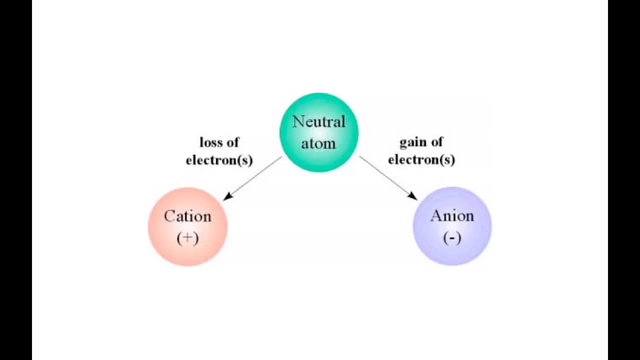 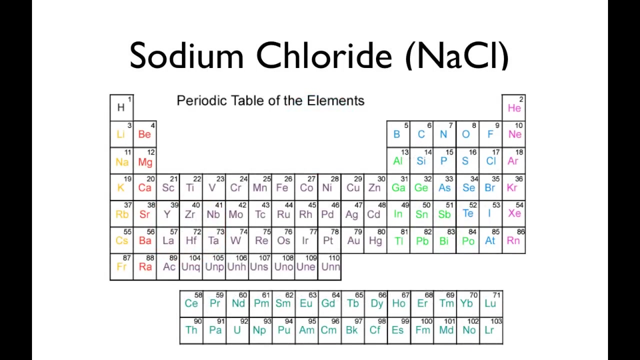 That is a positively charged ion. On the other hand, some atoms will gain one or more electrons. They also become ions, But they will gain a negative charge and we use the term anion to represent that. If you've worked with batteries, of course you're familiar with these- Cathodes, anodes, all the same thing. So the key is that these opposite charges attract each other. That's where the bond is. So let's look at the classic example of the ionic bond. Textbooks act as if there is only one example, but we'll look at it. 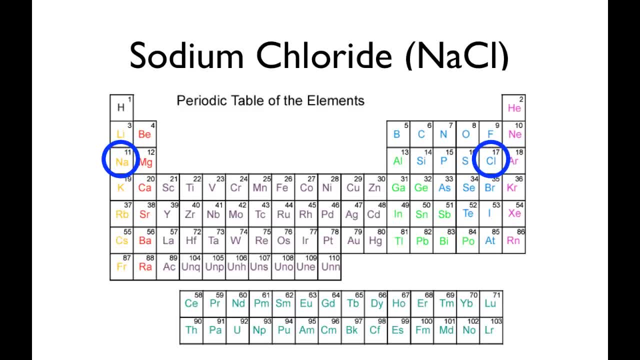 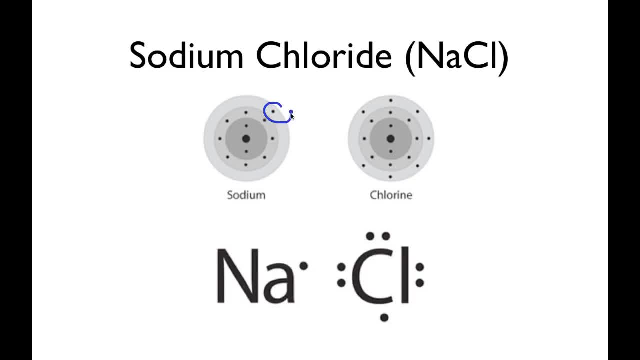 Sodium and chlorine. You notice they're at opposite ends of the periodic table. What we've got here is a scenario where sodium- remember the electrons- fill from the inside out and it's got a valence shell of one electron- one lone electron. This is not a happy situation. Meanwhile, chlorine has seven valence electrons and would like to have eight. It would like to feel like a noble gas, So it is also very unhappy. But when sodium and chlorine get together, something really cool can happen. 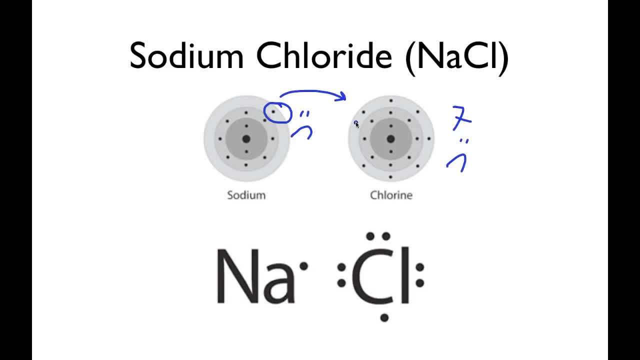 Sodium can lose that one electron. Look what happens now. Now its second shell. this shell right here is full, So sodium is happy. Meanwhile chlorine gains an extra electron. It then has a full valence shell also, So it becomes happy, Everybody's happy. 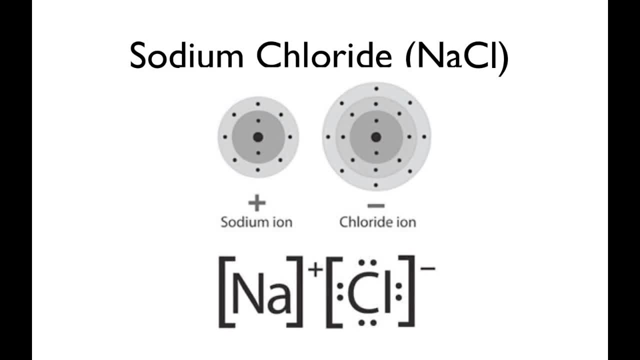 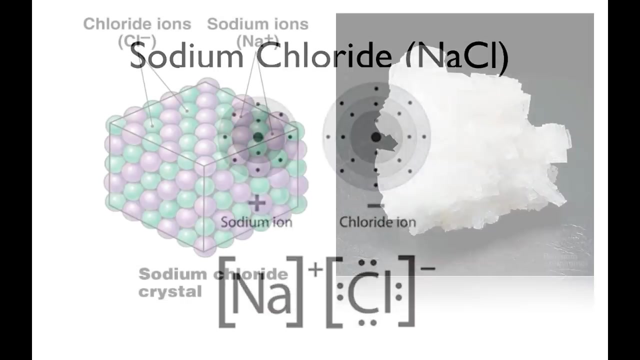 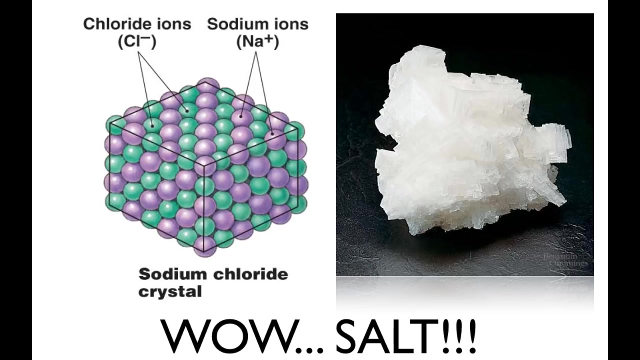 Now the thing is, don't forget, though, that sodium now has one less electron than it has protons, while chlorine has one extra electron compared to the number of protons. That's where those charges come into play. So now you notice that this is not an atom anymore, It's an ion. It has a charge. Specifically, it's a cation. Chlorine is also an ion. Specifically, it's an anion. It is the attraction between these two opposite charges that holds sodium and chloride together, And you make salt. I know it's just incredible how you make salt. It's so exciting. It's extremely stable, because sodium and chloride really like to hang out together. 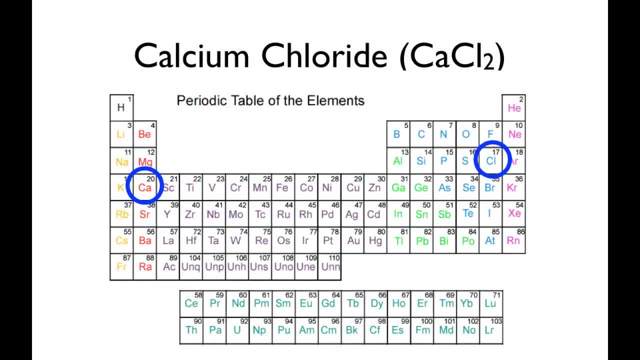 And you can see why Opposites attract. If you look at another example: calcium chloride. Now, if you recall, this group has two valence electrons And of course chlorine still has seven. So you might already start to think: hmm, if calcium has two electrons in its valence shell and it could get rid of those, that would also make it stable and happy. 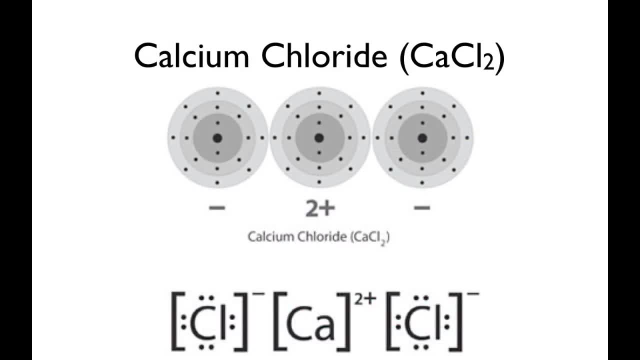 So all you've got to do in that case is bind with not one but two chloride ions in order to achieve that stability. So calcium gives up its two outermost electrons, One to this chloride ion and one to this chloride ion, And the whole thing is held together in a very stable configuration. 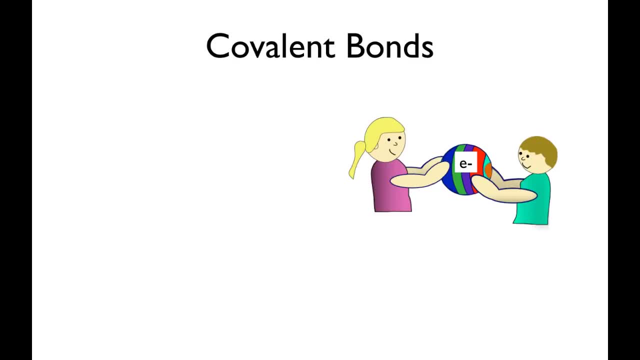 That's calcium chloride. So sometimes electrons are not taken but rather shared. When that happens, we refer to the sharing of electrons as a covalent bond. But immediately you might start to think: you know, is sharing always equal? Well, in humans, certainly, sometimes it is and sometimes it's not. 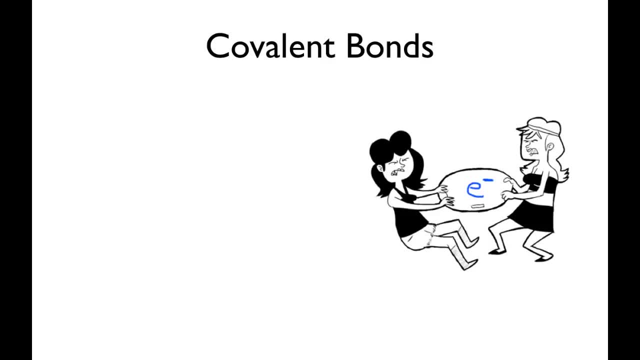 The same thing is true for atoms. So sometimes the atoms exert equal pulls on the electron And we refer to that kind of a bond as a nonpolar covalent bond. We'll see why in a little bit. Sometimes one atom has a stronger pull. 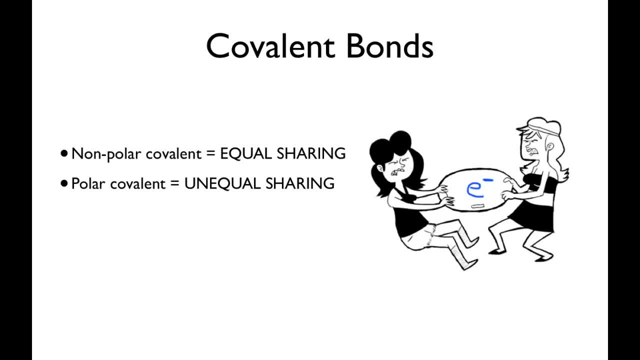 It wants the electrons more than the other. So it kind of the electrons will kind of play favorites because one atom is so much more desirable than another. How do you know who wants the electron more? How can you predict that? I mean, how would you ever know such a thing? 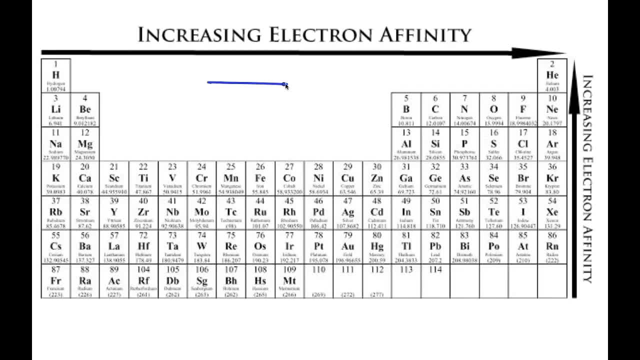 Oh my God, it's on the periodic table. It turns out that as you go across from left to right and as you go up, you have increasing electron affinity. That means how much any given atom wants electrons. They want electrons so badly the more you go towards this corner. 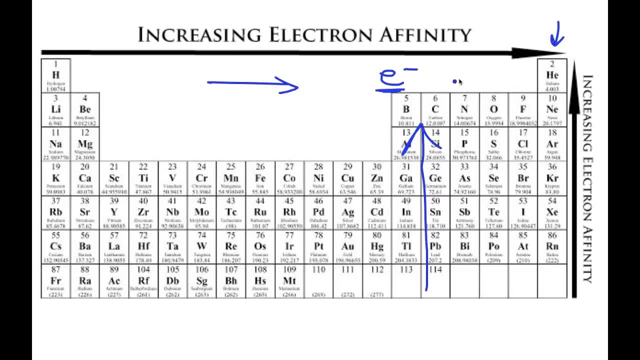 Remember excluding the noble gases, because they're already happy already. So who's at the top right corner? Oh my gosh, it's fluorine. Fluorine is the most important thing. Fluorine is the most electron desiring atom in the whole periodic table. 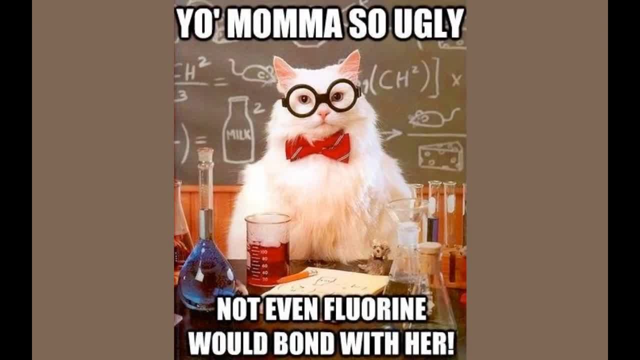 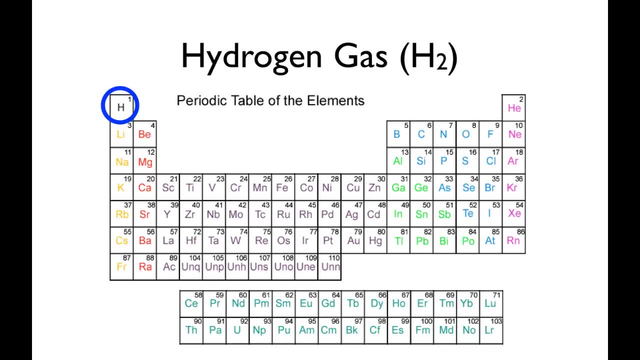 And if you know that, then this joke is actually funny. Okay, very geeky. So let's look at some covalent bonds, and we're going to look at the first one, hydrogen gas, which I actually showed you in the first video in my chemistry concept series. 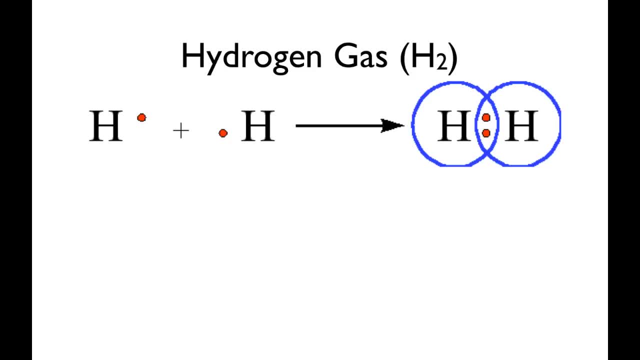 Hydrogen is the smallest atom. It has one electron, and its valence shell would like to have two. So one thing that hydrogen can do is get together with another hydrogen atom and share its valence- It's electrons. So each one shares the one electron that it has. 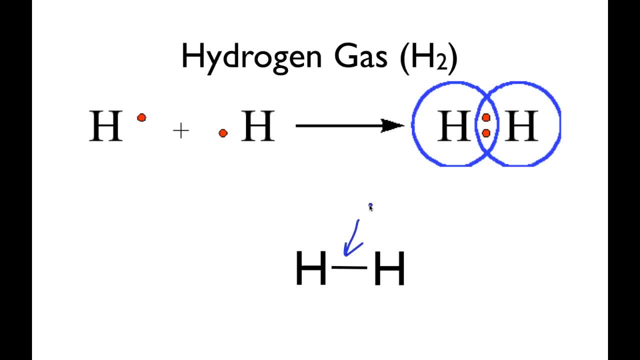 This is a typical way that we draw it, and when you see this little line, this means one pair of electrons being shared. Okay, So that's what those lines mean. You're going to see that all over the place. Now, it turns out, you can share more than one pair. 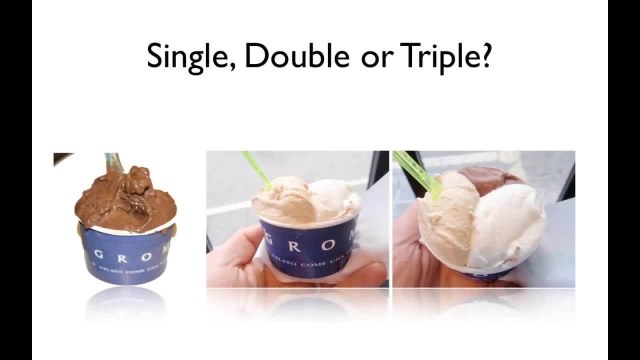 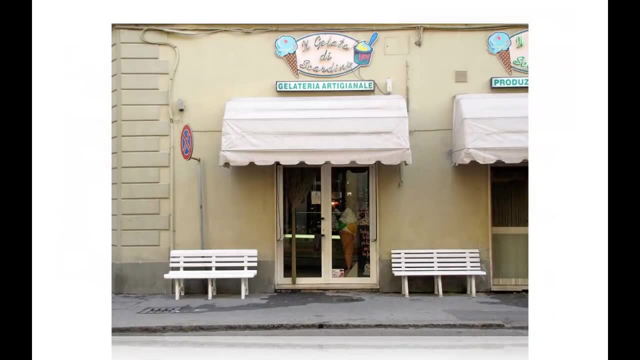 So you can have a single, as we just saw, but also a double or even a triple bond. Oh, I love gelato, Don't you love gelato? This is a reason to go to Italy. If you go, make sure that you look for this word: artigianale. 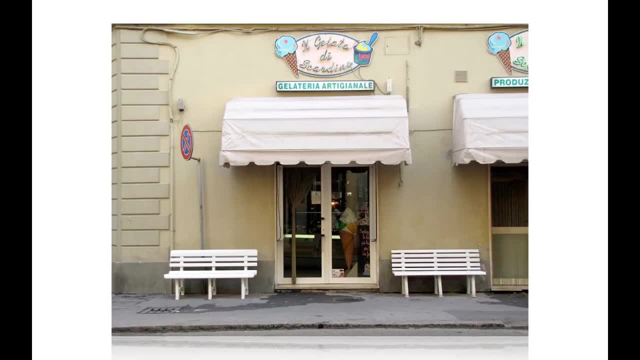 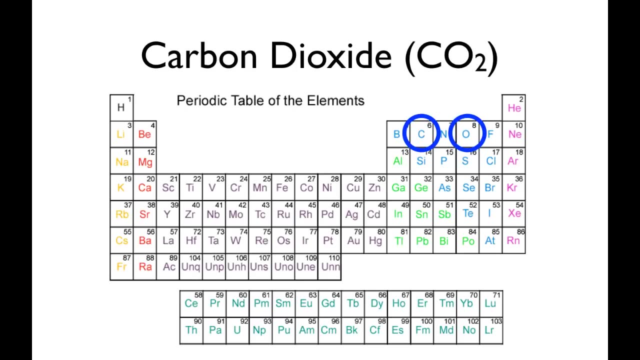 which means that it's actually handmade. If you're going to eat gelato, that's the only way to go. Sorry. Back to covalent bonds, We're going to look at carbon dioxide. So carbon, you recall, has four electrons in its valence shell. 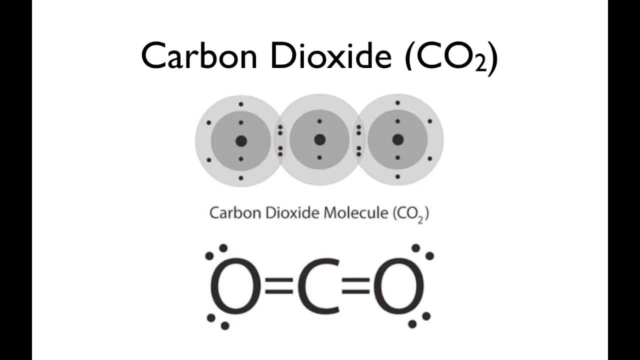 Oxygen has six. So in order for this molecule to be stable, you need to share more than one pair of electrons between the carbon and each of the two oxygens. So this means that with these two lines right here, that represents two pairs of electrons being shared. 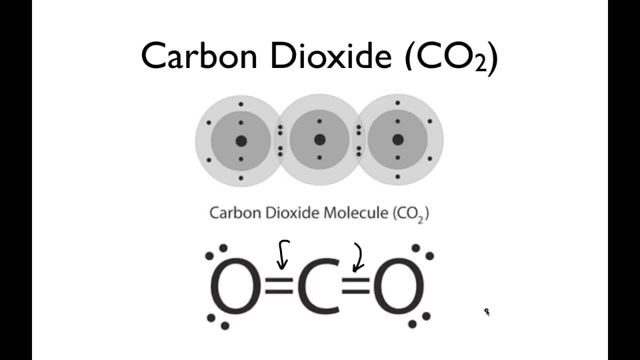 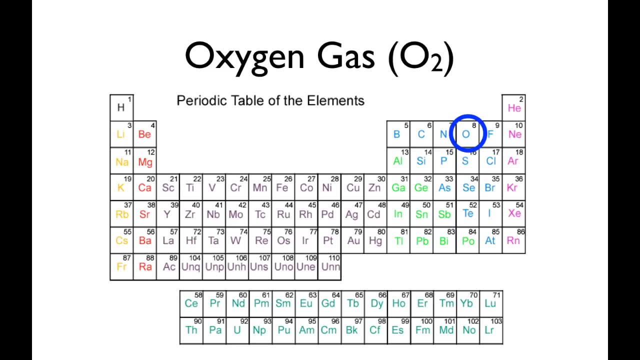 And these two lines here represent two pairs of electrons being shared. And now, if you count up all the electrons around each atom, everybody is happy. They all have eight electrons in their valence shell. What about oxygen gas? Oxygen has six electrons in its valence shell. 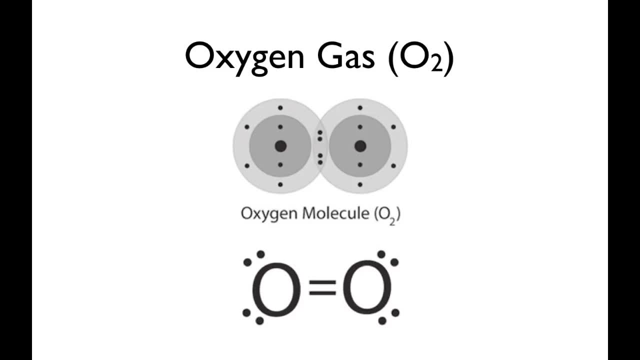 So if two oxygen atoms come together, in order for them to have the full octet, they also need to form a double. Okay, And now, if you count around for each of the oxygens, this line represents two. This line represents two for four. 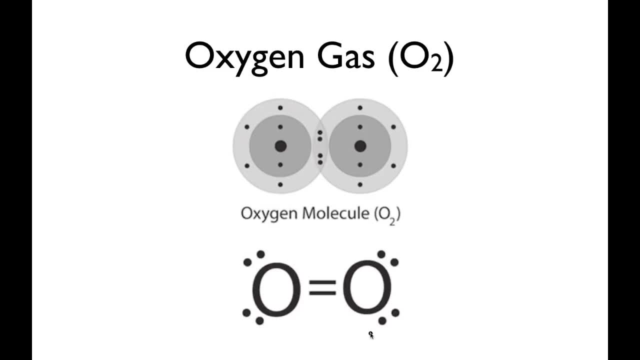 Then you have five, six, seven, eight. Same thing for this guy, So everybody is happy. Okay, Let's look at one more. How about nitrogen gas Now? nitrogen has five valence electrons, So for nitrogen to form covalent bonds with another nitrogen, they need to share three pairs. 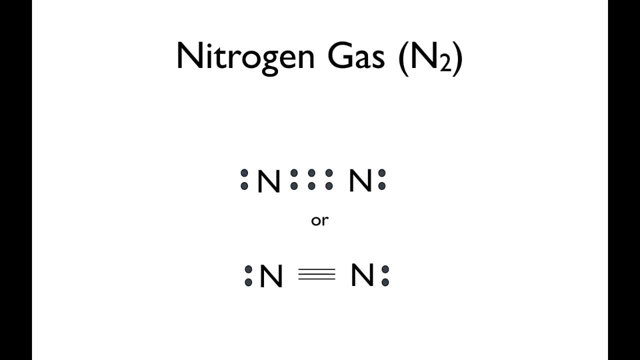 So two nitrogens will come together and form a triple bond. So covalent bonds represent sharing of electrons And so far all of this sharing that we have looked at is equal. These are nonpolar covalent bonds. What if the sharing is unequal? 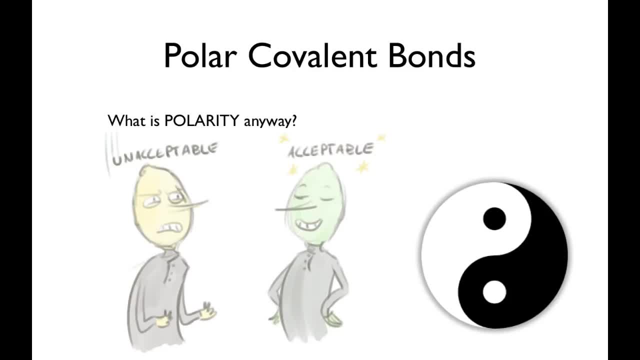 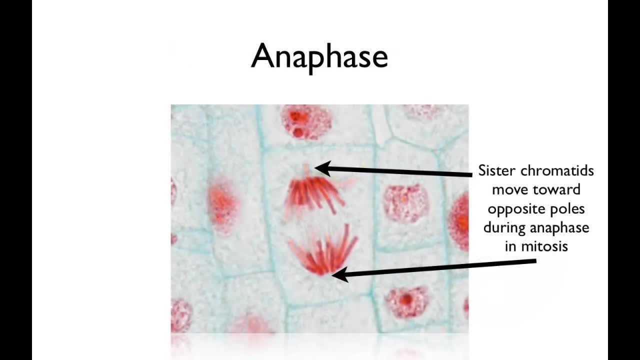 We've got to talk about this term, polarity, And hopefully the term polarity makes you think about dualism or something where there are two sides that are different. In biology, if you think about mitosis and you know about the opposite polarity, you're going to think about the polarity of a cell as it prepares to divide. 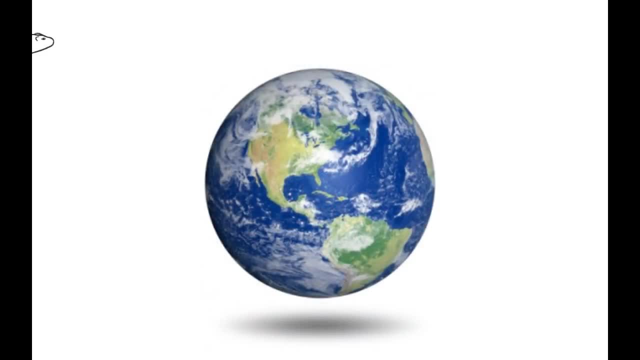 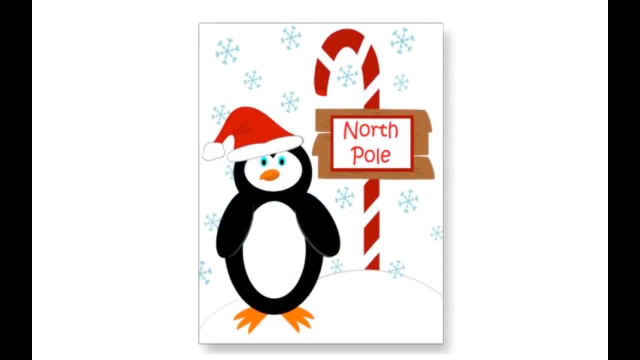 That could help. Most people know about the poles on the globe. of course. We have the North Pole with polar bears And we have the South Pole with penguins on it. That's a pretty good example. Now, if you didn't know that and you thought there were penguins, 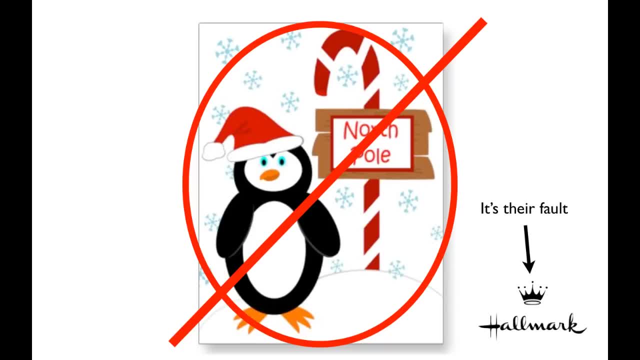 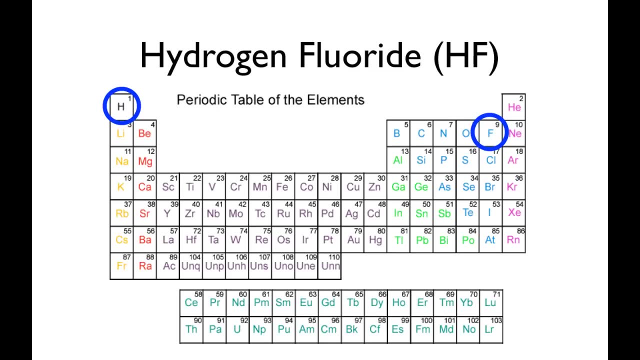 at the North Pole. don't feel bad, It's not your fault. It's because Hallmark puts penguins on the Christmas cards And with Santa. it drives me crazy. Okay, Let's look at a situation where electrons are not shared equally, as in the case of hydrogen. 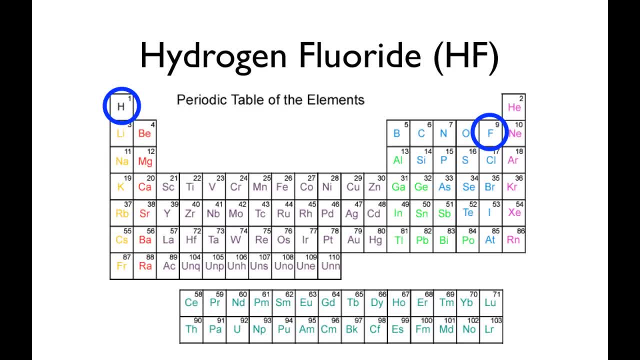 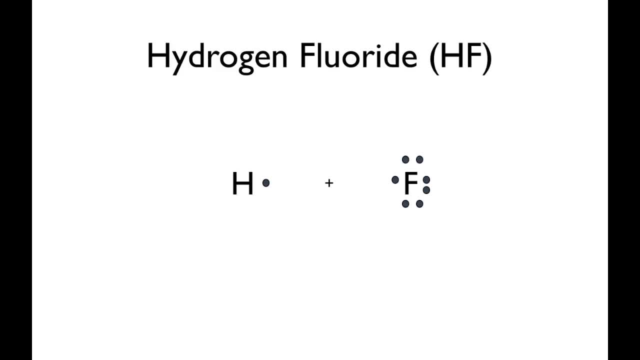 Hydrogen fluoride. Remember, fluorine wants electrons more than anybody else on the periodic table. So let's look at hydrogen and fluorine as they come together. Hydrogen has one valence, electron. Fluorine, of course, has seven. 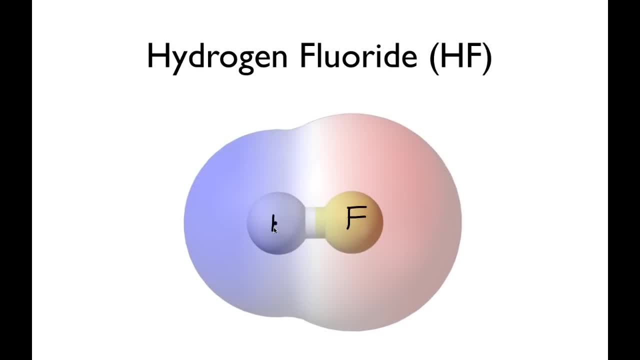 And when they come together. so this is fluorine and this is hydrogen, And this diagram is supposed to represent the fact that fluorine has such a great pull on the electrons that the redder color represents the more negative side And the blue represents the negative side. 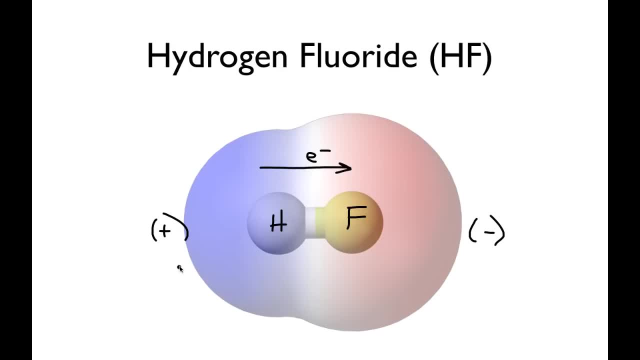 And the blue represents the more positive side of this thing. Now, these are not electrical charges. This is not an ion. This is still a covalent bond, But it's polar, So it means that one side of the molecule is more negative. 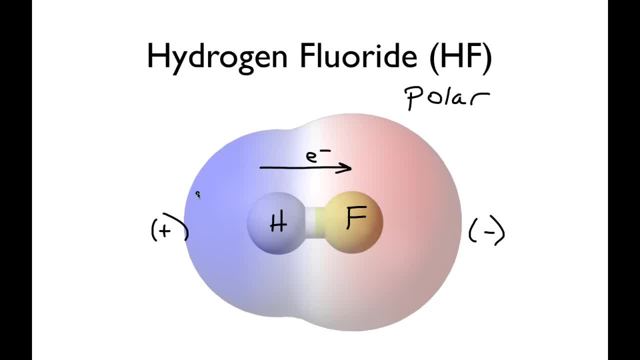 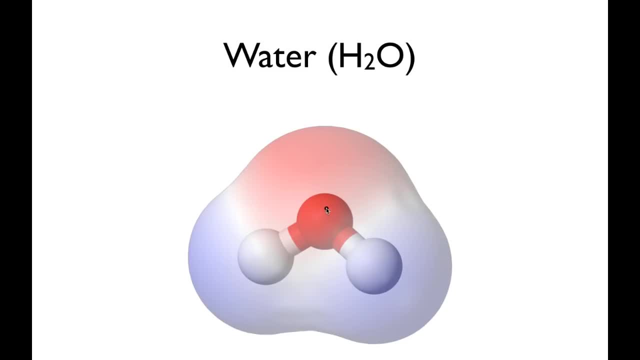 The other side of the molecule is more positive, So we call this a polar covalent bond. Another classic example of polar covalent bonds: water. Here's the oxygen And these are the two hydrogens, And the oxygen exerts a much greater electron pull. 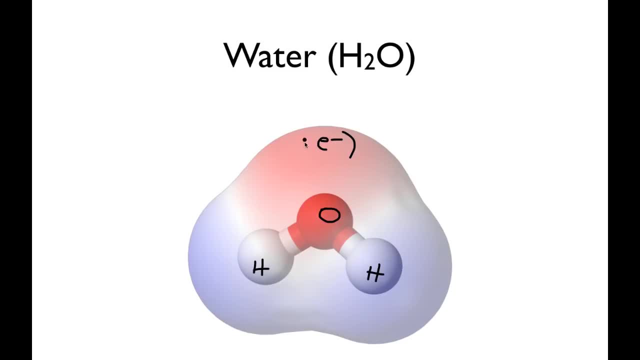 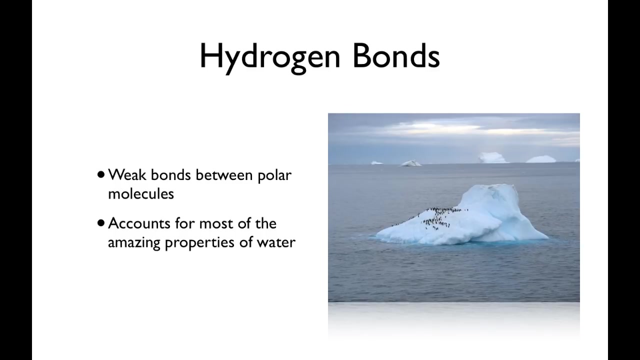 than the hydrogens. So the electrons prefer to hang out more on this end. So it makes this end, the oxygen end, slightly negative. The hydrogen end is slightly positive And that's why water is polar. It turns out that hydrogen bonds are kind of related to this. 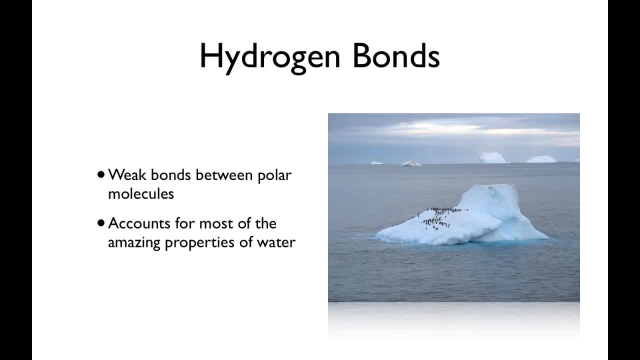 Hydrogen bonds are weak interactions between slight negatives and slight positives. Even if it's slight, opposites still attract. And it's actually hydrogen bonds that account for all the amazing properties of water, the fact that water holds so much heat. It has a high vaporization. 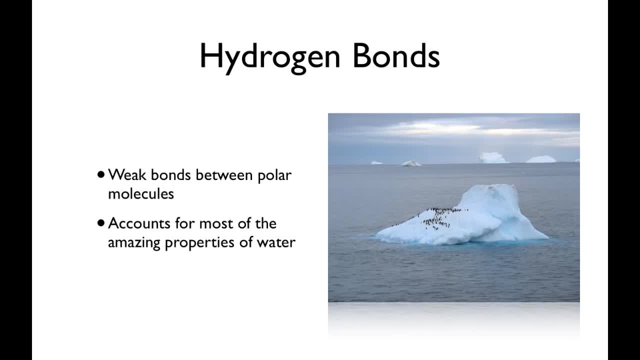 The fact that ice floats. I mean, you probably don't think about this too much, unless you are a penguin, But it's something that other substances don't do right. The solids are always more dense than the liquids, And this is all because of hydrogen bonding.